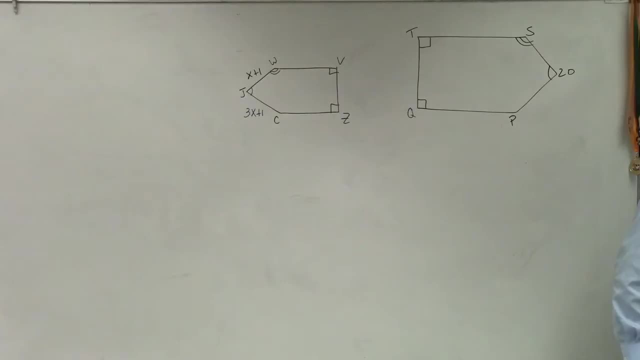 on this problem. it actually does give us the congruency. Actually, well, we don't even need the congruency, But you guys can see that if I was going to say that these triangles are congruent, triangle JWVZC is similar. I'm sorry, not triangle quadrilateral Or not even quadrilateral. 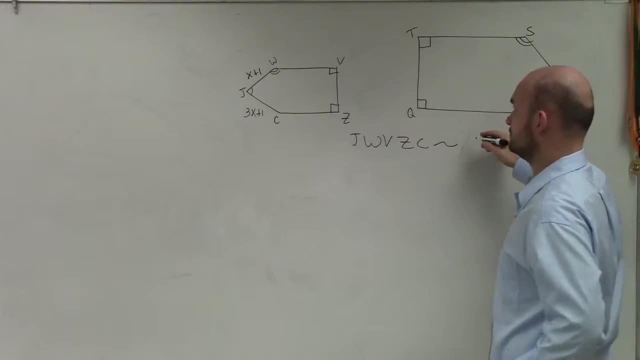 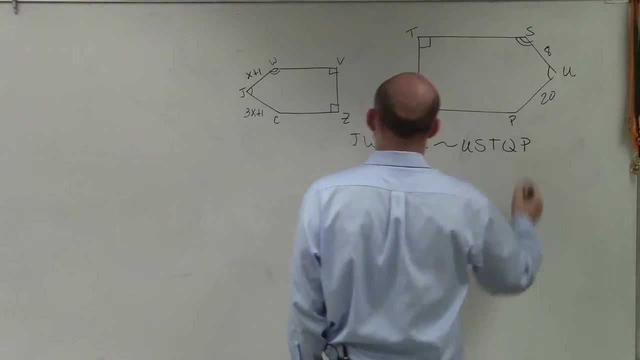 Pentagon To Pentagon. What the heck did I do? That's 20.. Sorry about that. That's 8.. Yeah, the side is 20.. Sorry, Sorry, I forgot. I didn't mention all that, So those are going to be similar to each other Now. 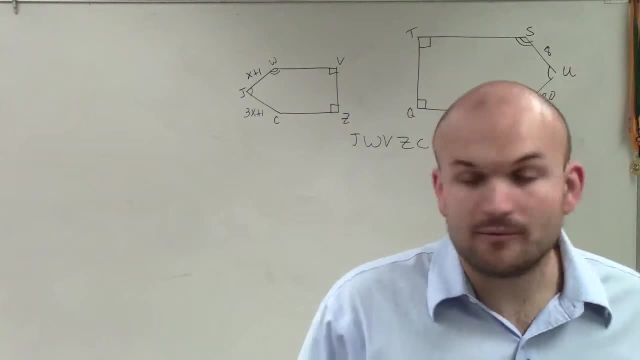 so what I want to do is rewrite sides. all right, That way I'm going to be able to do it. So I'm going to do it, So I'm going to do it. So one thing that we can write a proportion for, because we can't solve anything of similarity. 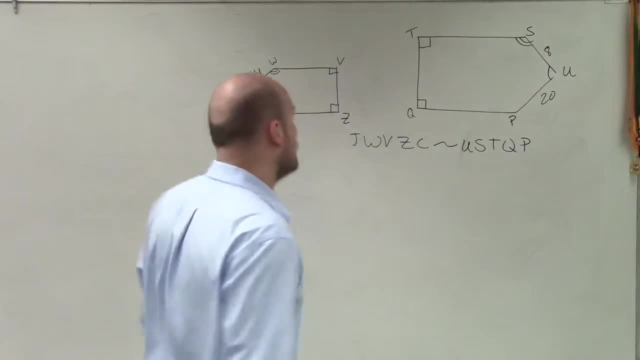 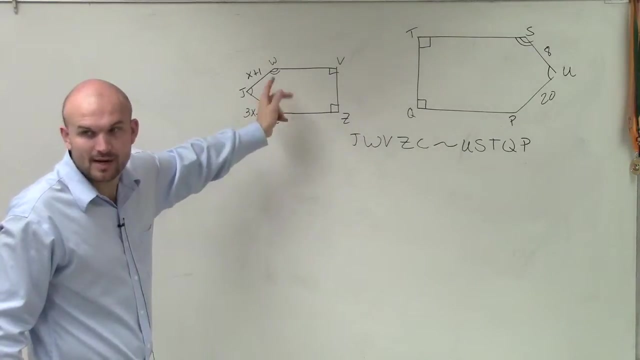 unless we have a proportion, all right. So one thing I want to look at here is I? so if you guys see, here's my similarity statement, right. I want to be able to see what side is JW similar to that I can write a proportion for. So JW is similar to what side over here? 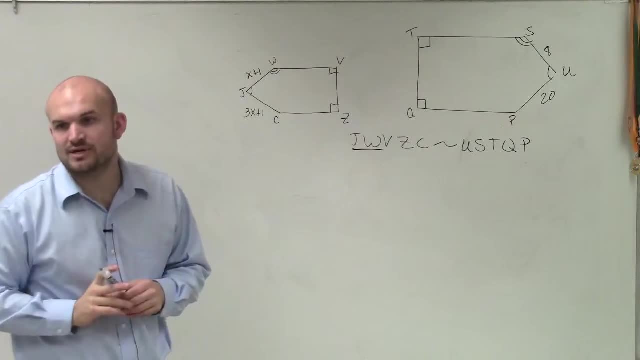 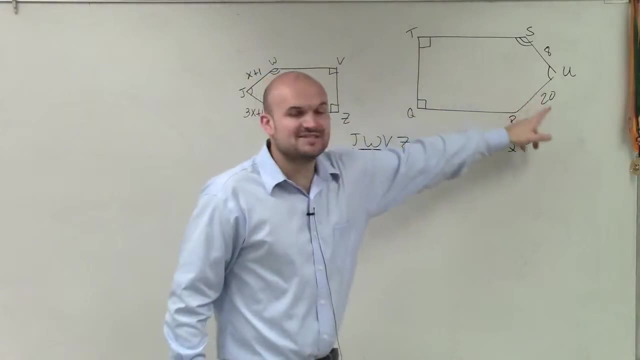 U-S or S-U. Which one is it U-S? I think it's S-U. Right. So J is to W as U is to S Layla, you need to remain always facing forward. Put your knees on your desk, fully on your desk. 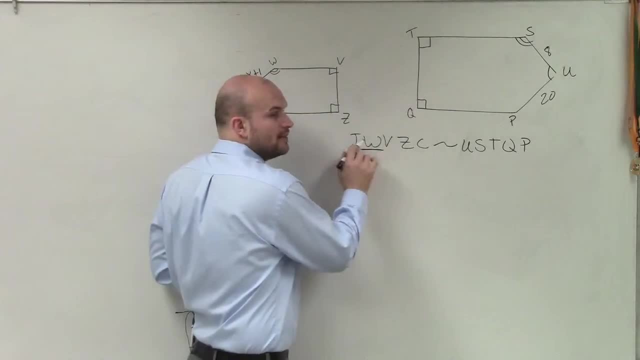 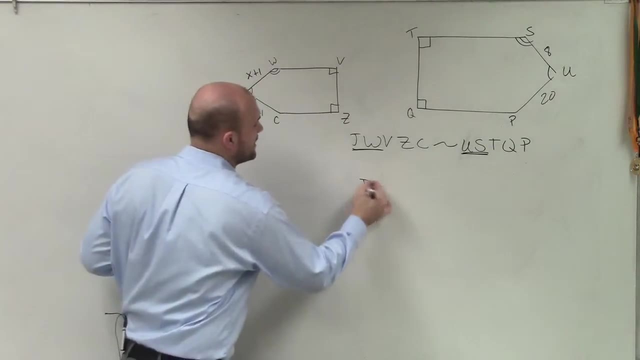 and stay that way, please. Thank you. You can also look at it this way: JW is the same as US, not SU US. make sure you're just going in the same direction. So I'll set up a ratio: JW is equal to US. 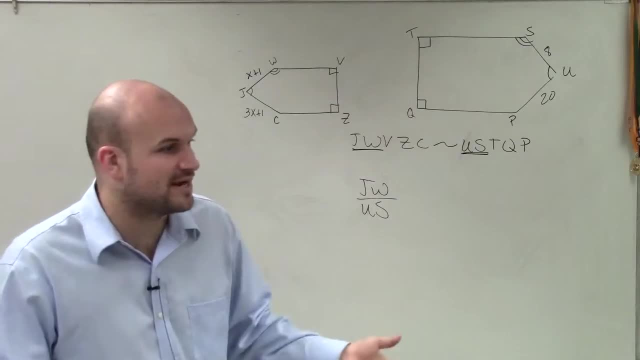 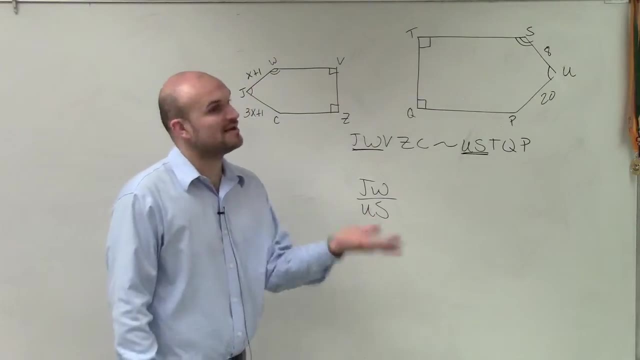 Now remember that's going to be the same ratio for all the other side's ratios, that we can find right Ratios, But let's go and find another one that we can set a proportion, Because once we have a proportion we can solve. 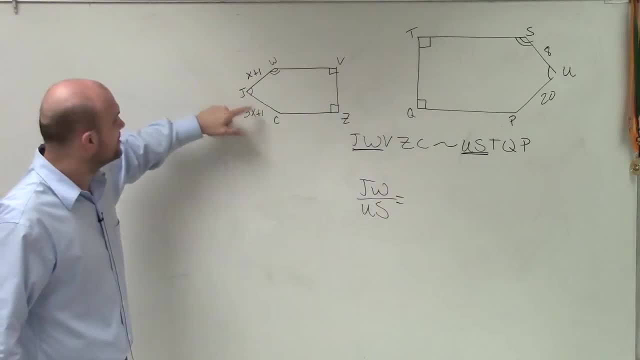 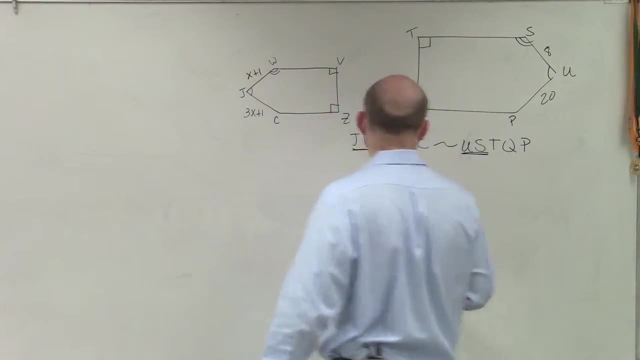 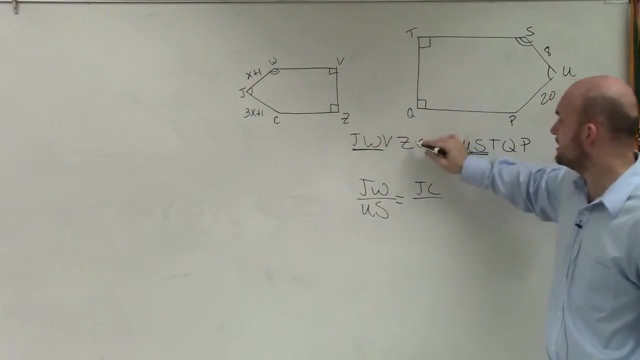 So I also notice here I have one which I could call that JC, which gives you 3C. So JC is similar to what other side over here? U-T. U-U-U-P Right. Think about it this way, JC, right. 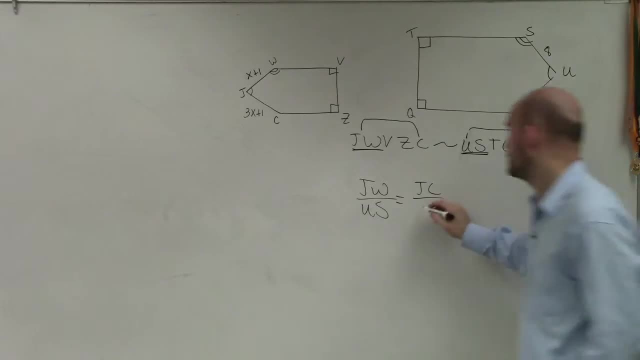 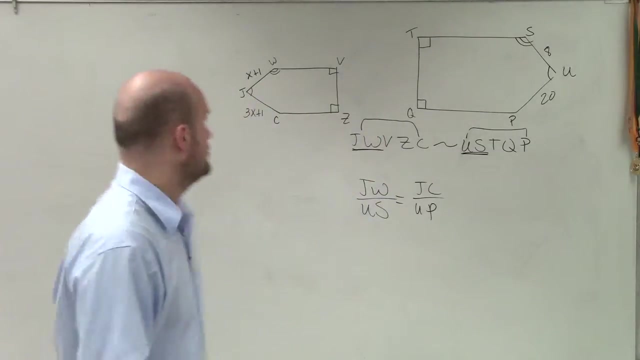 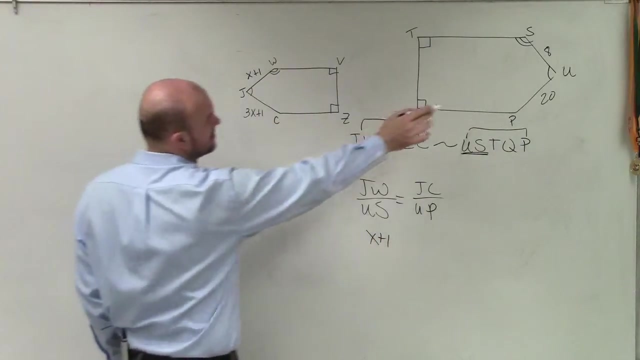 J to C is the same as U to P. All right Now, ladies and gentlemen, what I want to do is now, let's plug in what we know. So we know that JW is x plus 1.. We know that US is 8, which is equal to JC, which is 3x plus 1.. 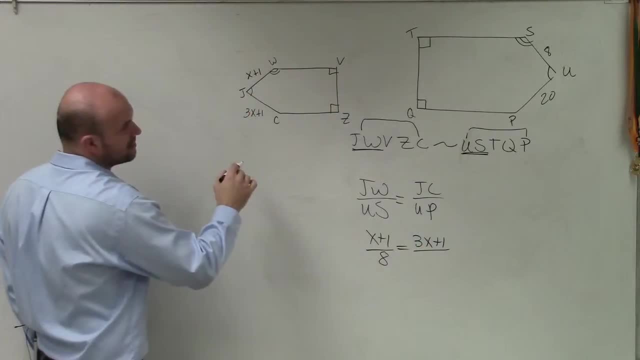 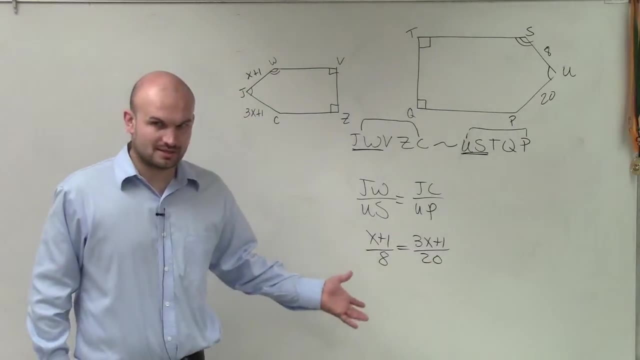 What is 3x plus 1? And UP is 20.. What I'm doing you do need to understand, or you're not going to be able to understand how to take a test or do the homework or anything else, on your own. 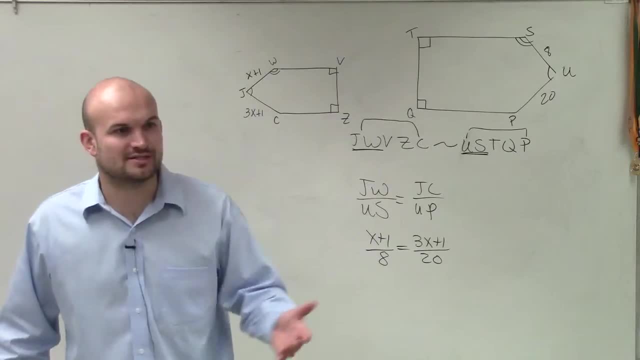 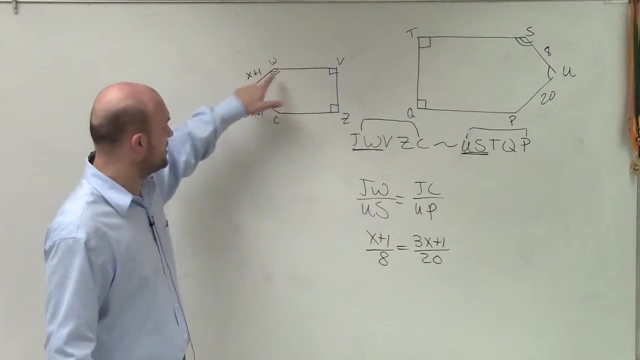 Then you're just a robot doing exactly what I need you to do, And then you're just not going to be able to pass anything else. So all I'm doing, John, is I just take in each value JW right here. 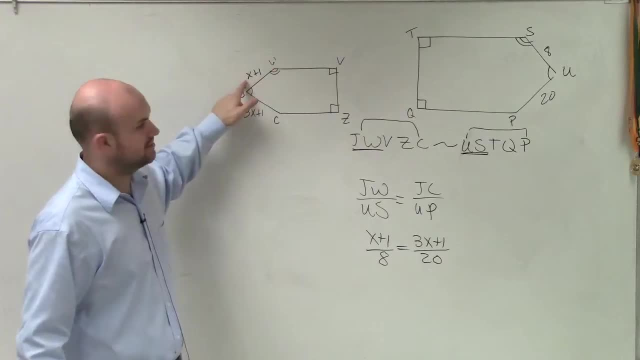 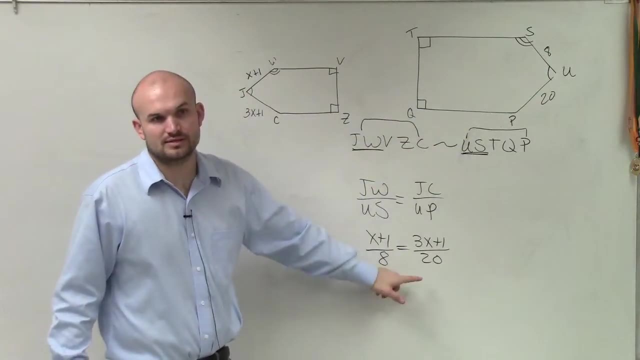 That value is x plus 1.. JW: x plus 1.. Then the next one, which is US. US is right here, The length is 8. So all I did was I plugged them in for their lengths. Now we go ahead and take our product, which is cross-multiplication products. 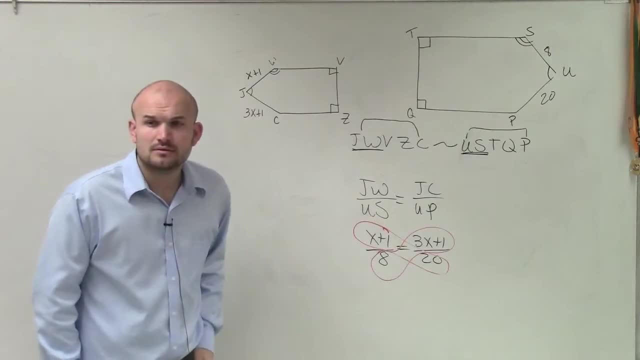 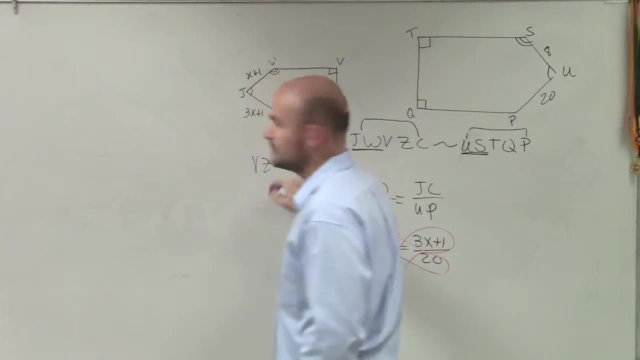 What do you mean? You want me to do some other sides? Well, no, I'm just asking why you chose those two. Well, because those are the two that have variables with them, right? I mean, what good is it going to be if I say what is vz? 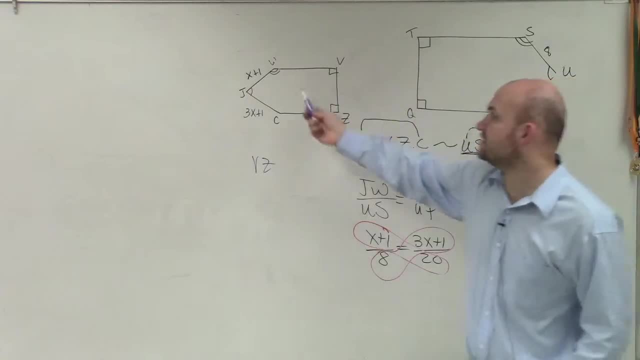 I don't even know any measurement on vz, See what I'm saying. So yeah, you want to use the one where obviously you have some variables of something to solve for. OK, Kiana, could you put your knees under your desk please? 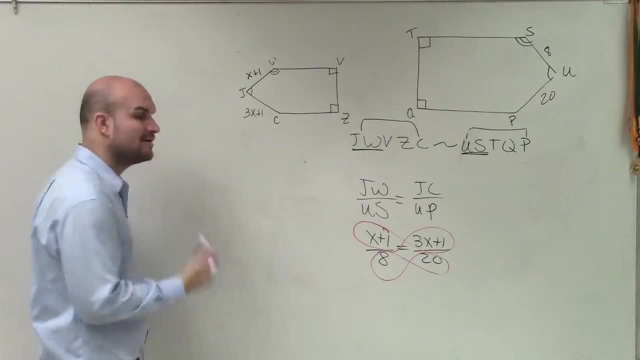 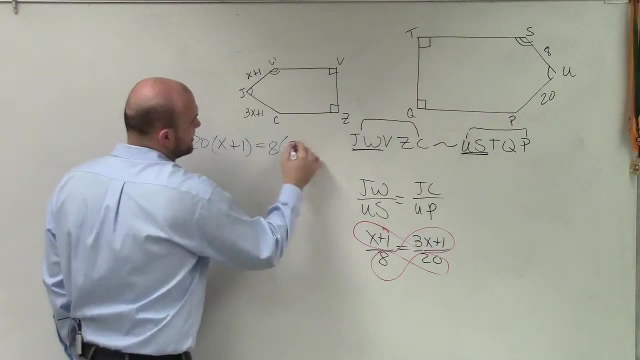 So now, yeah, you just go ahead and solve. So again, what I would recommend, guys, when you're doing this cross product, is do 20 times, 20 times x plus 1. Make sure you apply those parentheses. 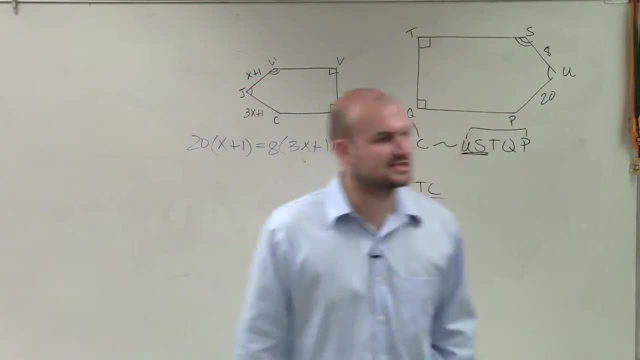 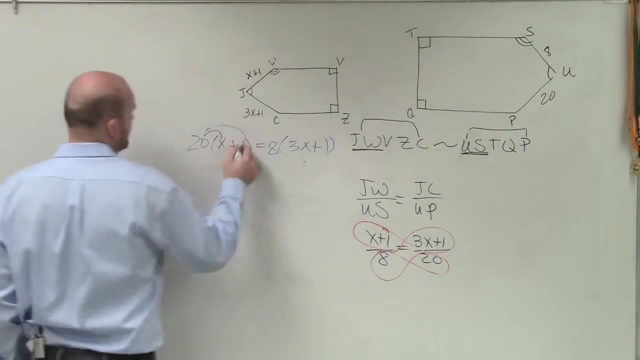 Because I guarantee you- the majority of you, this is where you're going to get stuck- is. you're not going to apply the parentheses in there And you're going to forget to apply distributive property, So What You don't want to.